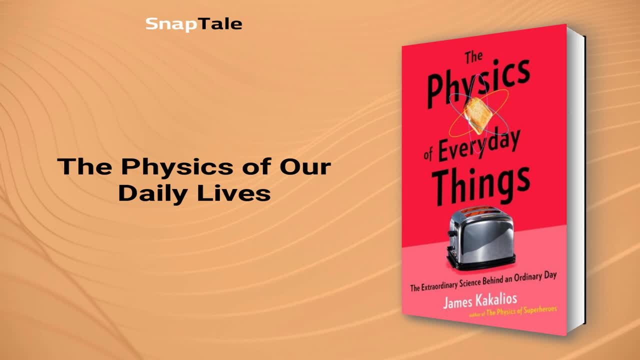 of the technology we use every day, from toothbrushes to touchscreens, In The Physics of Everyday Things. James Kekalios takes a look at the physics of everyday life. James Kekalios is a professor at the University of Minnesota and he paints readers on a physics-infused journey through a day in the. 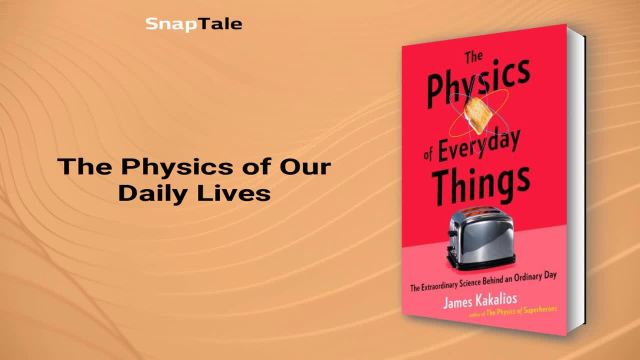 life. He starts by examining the technology we rely on each morning, from the electromagnetic waves used by our smartphones to the energy conversion principles at work in our coffee makers. Kekalios delves into the science behind the batteries in our toothbrushes, explaining 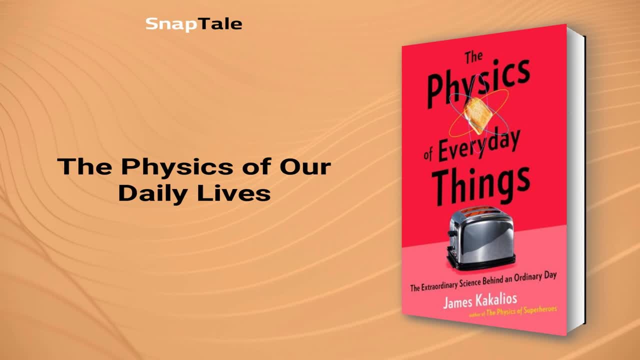 how transformers and alternating currents work together to keep our devices charged. He also explores the mechanics of the internal combustion engine and the technology behind GPS navigation and E-ZPass tollbooths. Moving on to our wireless devices, Cacalios explains how 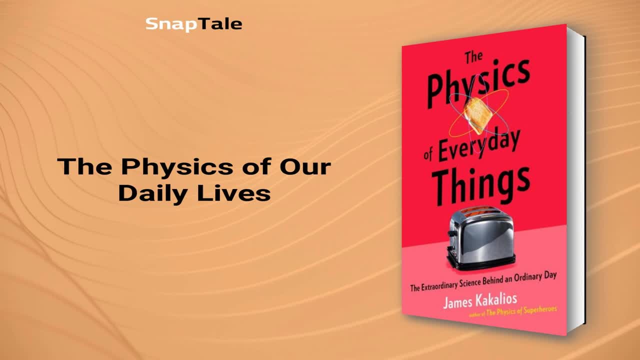 radio waves keep us connected to the internet, and how digital signals can transmit enormous amounts of data with little interference. The author also takes a closer look at medical technology, discussing how ultrasound can detect anomalies in our bodies and why touchscreens won't work with gloves. Throughout the book, Cacalios emphasizes the principle of conservation. 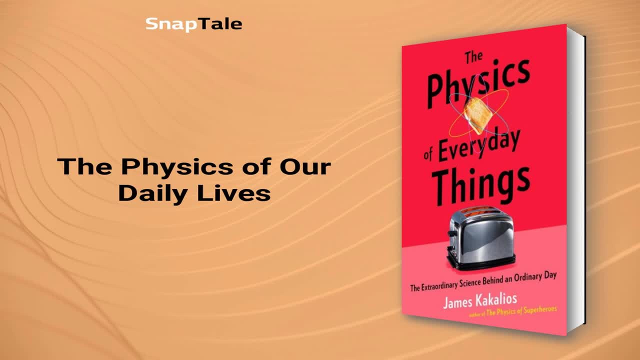 of energy which governs all aspects of our daily lives. He also highlights the basics of electromagnetism, demonstrating how electrical currents create magnetic fields and vice versa. Cacalios explores the physics behind noise-canceling headphones, illustrating how sound waves can be converted into electrical voltages and back again to cancel out incoming. 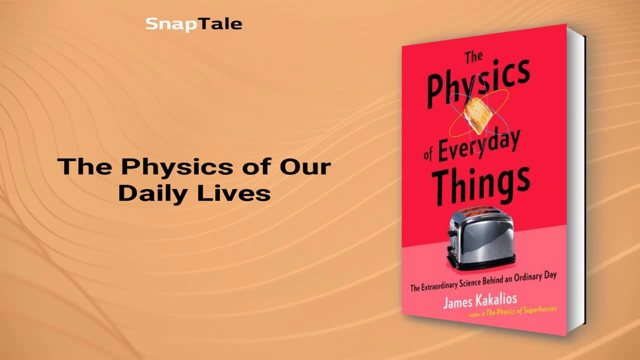 ambient sound waves. He also describes how photodiodes in camera pixels capture light and match colors, From the lift created by airplane wings to the microwaves used in airport body scanners, the Physics of Everyday Things offers readers an in-depth look at the physics that underlies 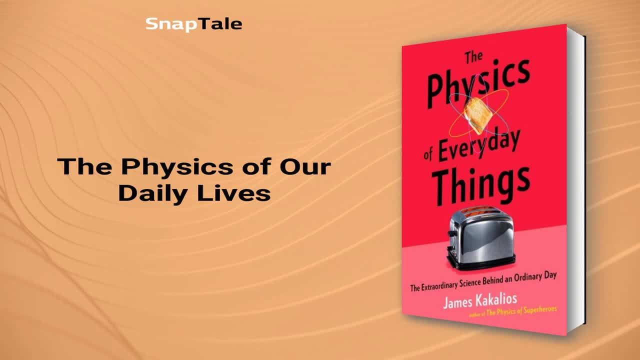 the technology we use every day, both old and new. Cacalios makes complex scientific concepts accessible and engaging, making this book perfect for anyone interested in the science behind our daily lives. Physics Enthusiasts Unite In The Physics of Everyday Things. Cacalios discusses how the world's most important 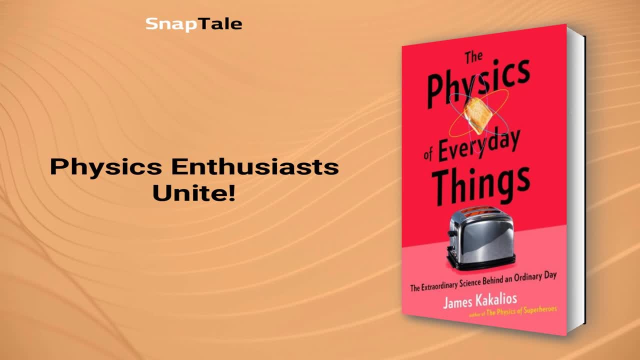 and most important things are important to us In The Physics of Everyday Things. Cacalios discusses how the world's most important and superheroes. James Kakelios employs a folksy approach to teach readers about the science behind comic book heroes. While some explanations may be oversimplified, Kakelios' love for physics.